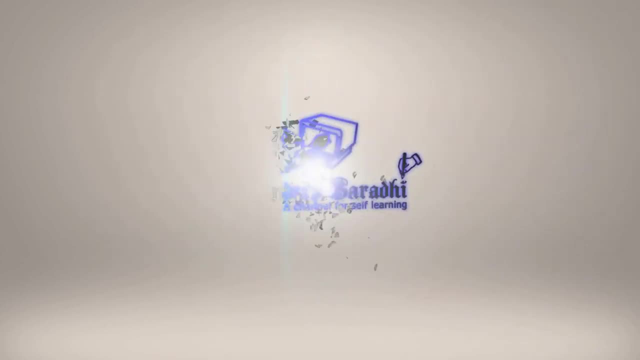 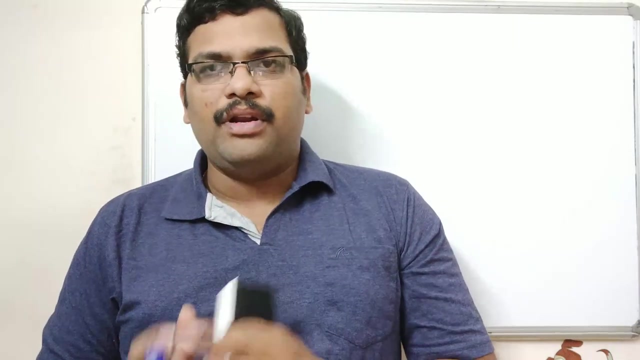 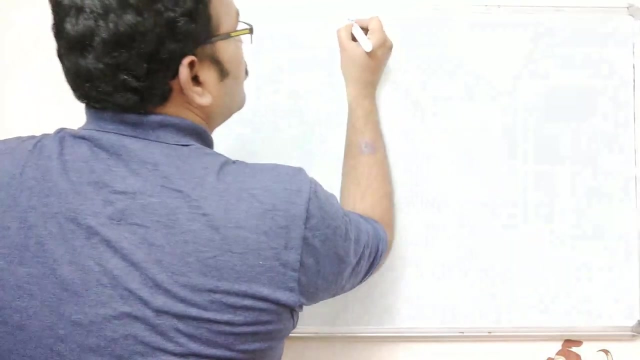 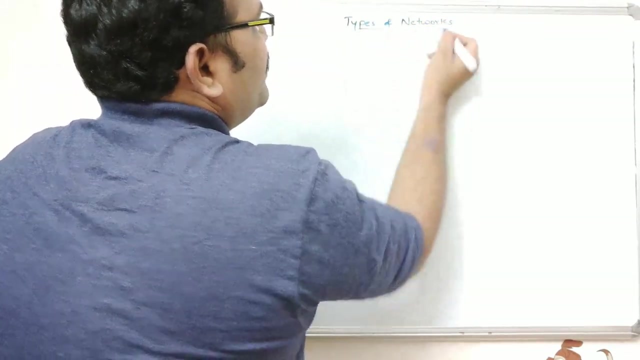 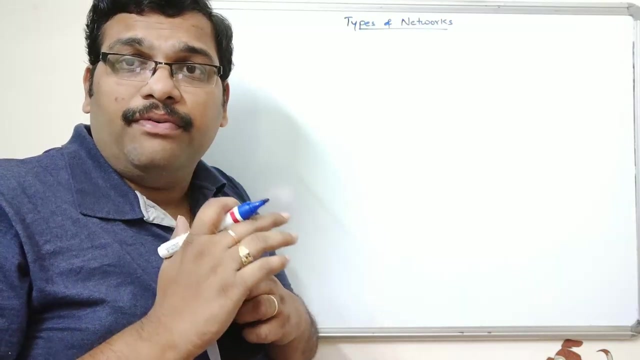 Hello friends, welcome back to our channel. So in the previous session we have seen the introduction to computer networks and in today's session we will go with another concept, that is, types of networks. So in the previous session we have seen what is the definition of a network. So definition of a network is a collection of or a connection of several computers is called a network. 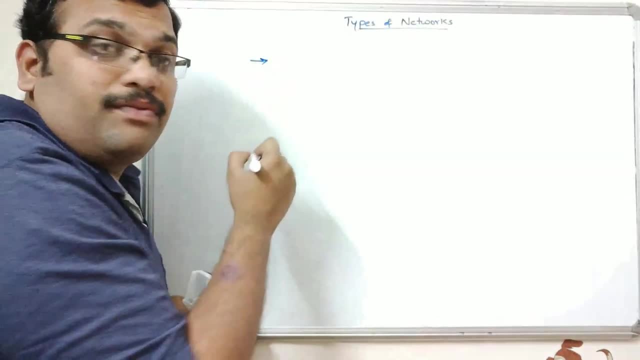 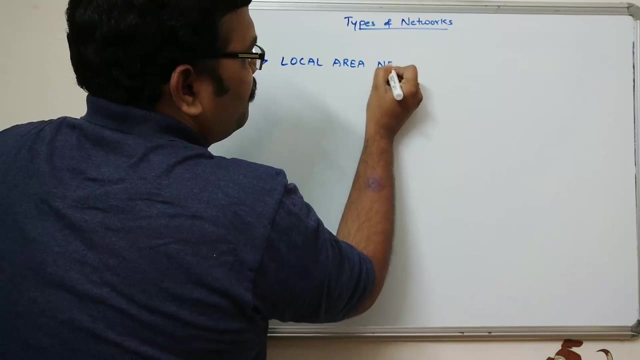 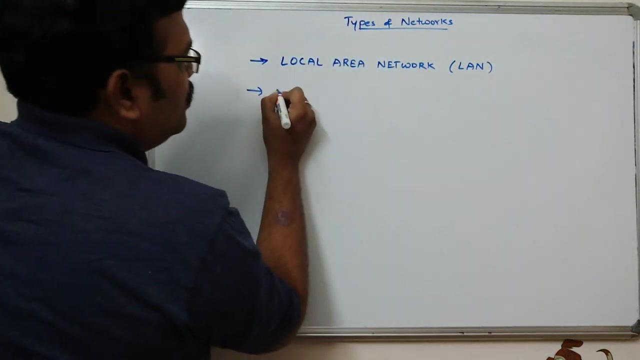 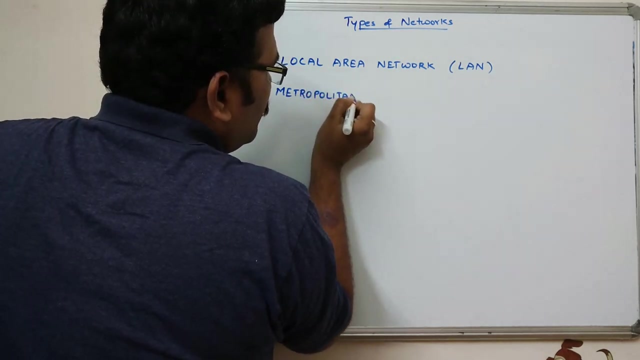 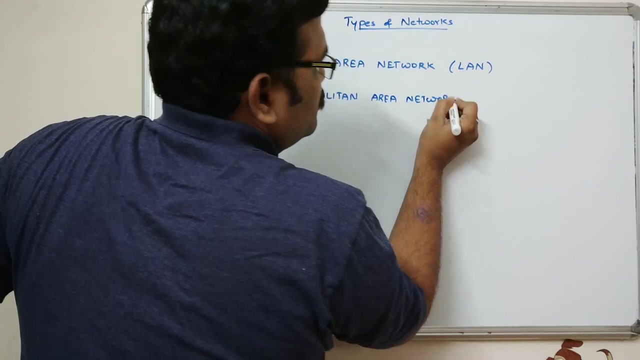 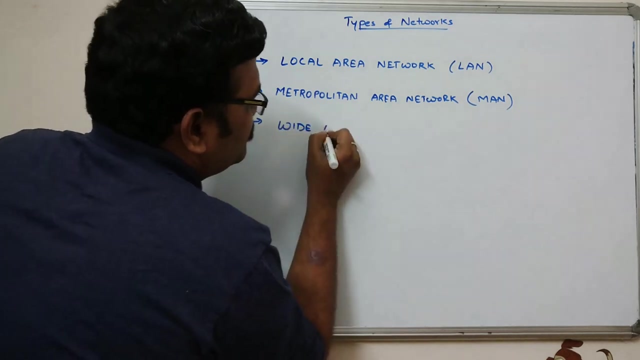 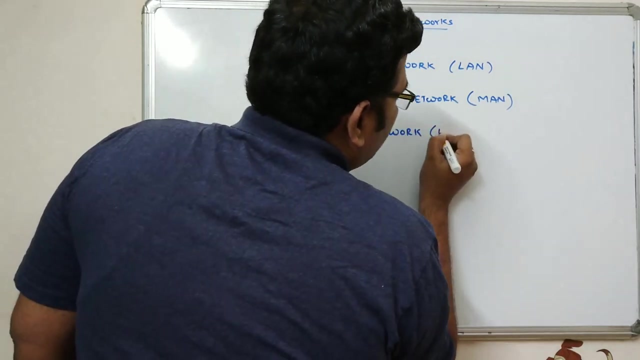 So here, majorly, there are three types of networks. One is local area network, which is known as LAN, METROPOLITAN NETWORK, Which is called as MAN WIDE AREA NETWORK, Which isلي memory space, Which is very well. 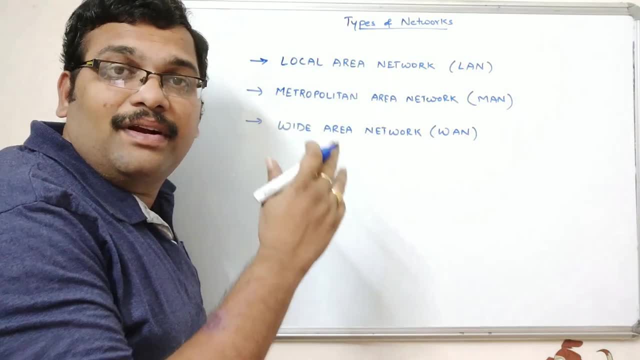 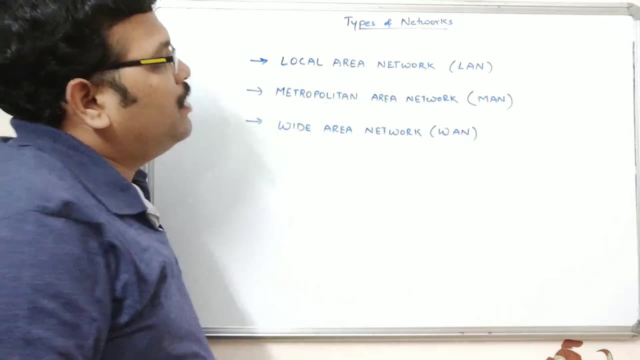 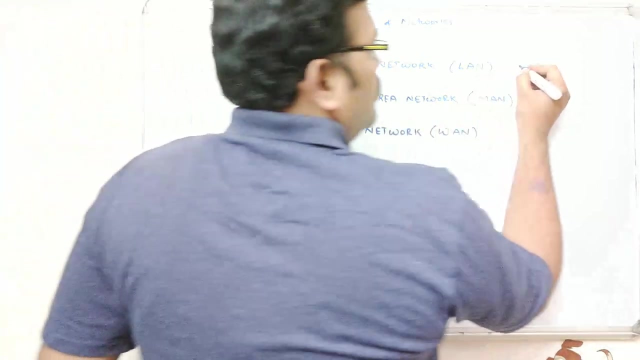 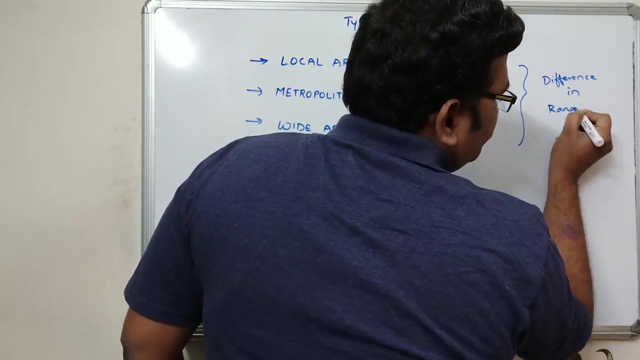 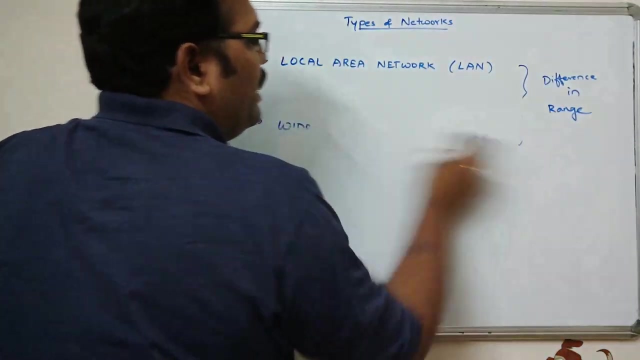 so these are the different types of networks, so different ways we can connect the computers. now we'll see one by one. so the main difference between all these three is the range difference in range right. so let us see one by one. first we'll go with the local area networks, so local, 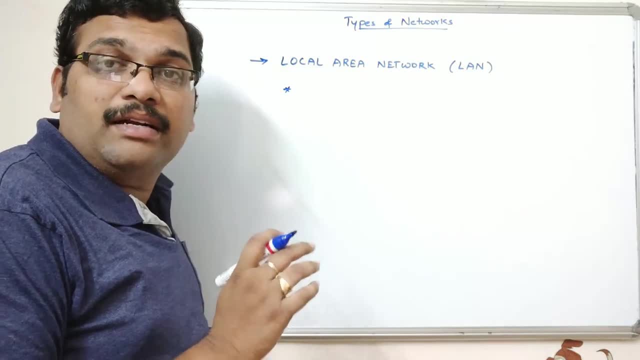 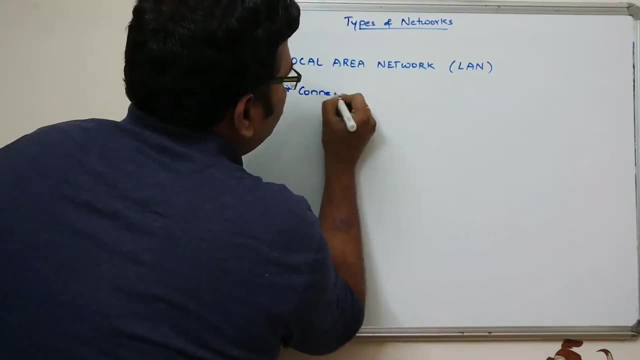 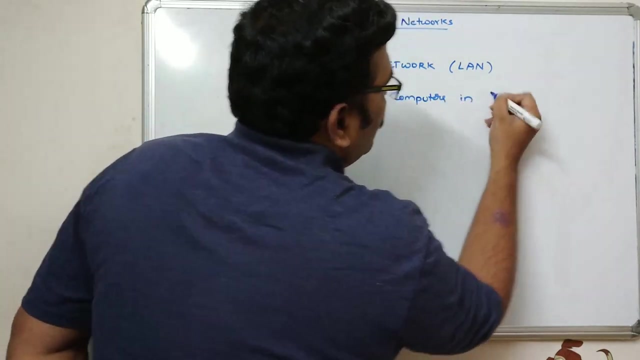 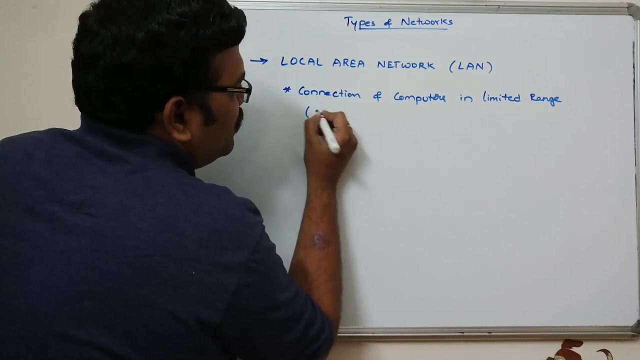 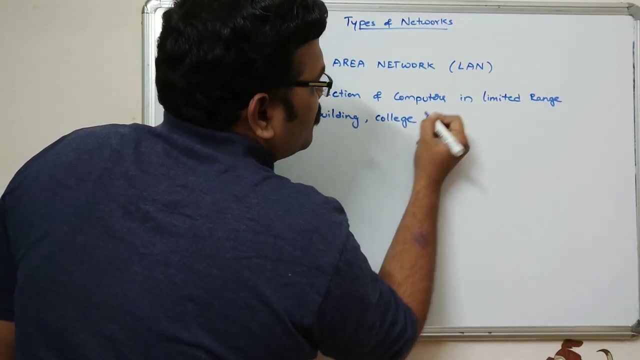 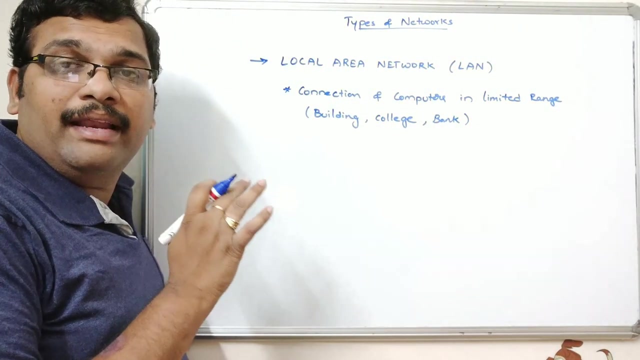 area network means the name itself indicates that computers will be connected in a specified range. so connection of computers in limited range in terms of I mean in a building or within the college, or within the bank, etc. so this is called the local area networks. right then, the main purpose of the local area networks is to 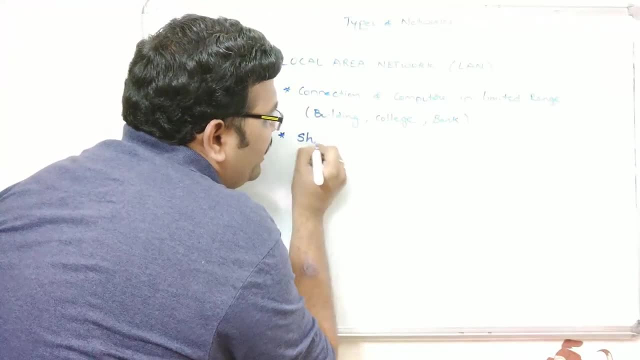 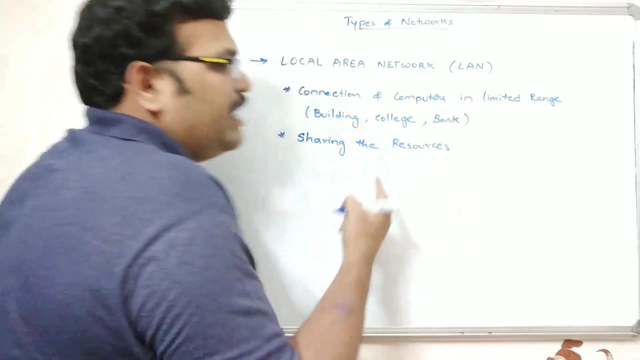 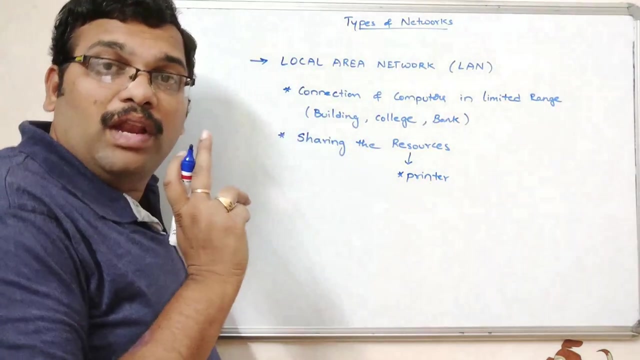 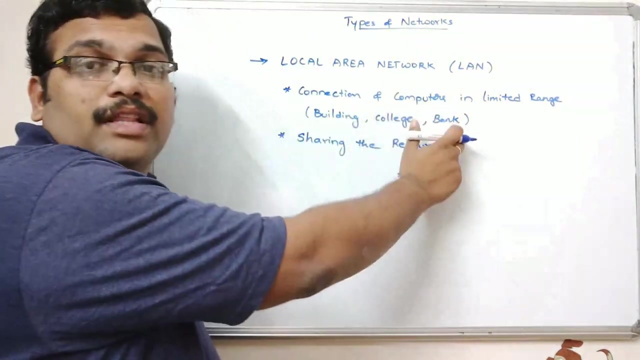 this land means sharing the resources, see. sharing the resources means the first one. we can use the printer. you can have a only one printer which can be shared among all the computers in the specified building or within the college or within the bank, so we can share the common printer. similarly, 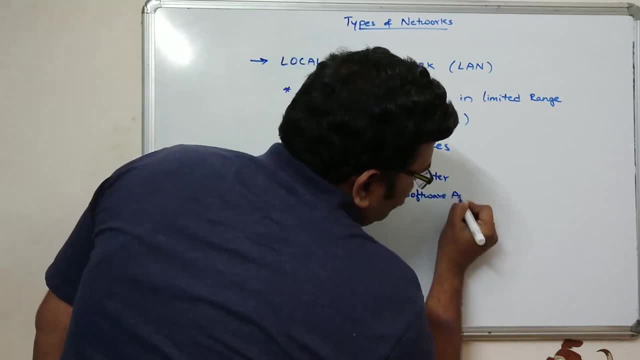 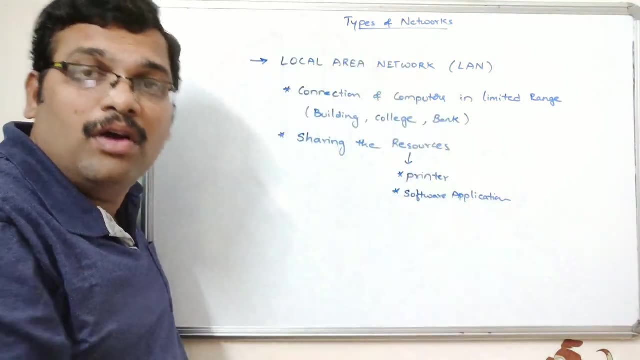 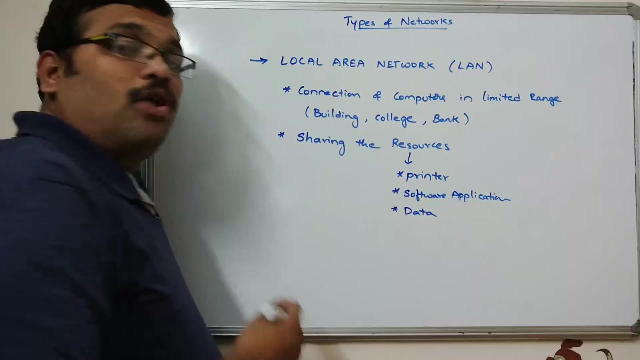 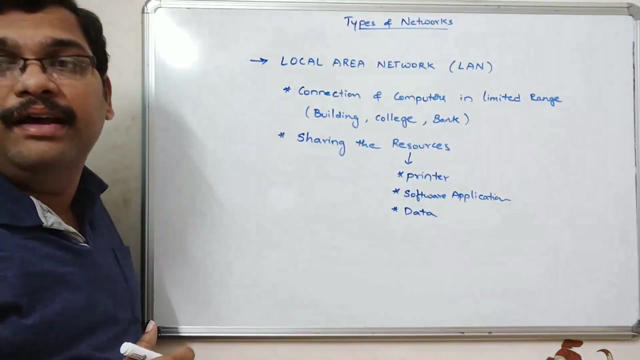 some software application, so an application can be installed in one system and that can be shared among a different computers in a local area network. and the third one is data. so this is common, so we can also share the data among all the users in a local area network. and 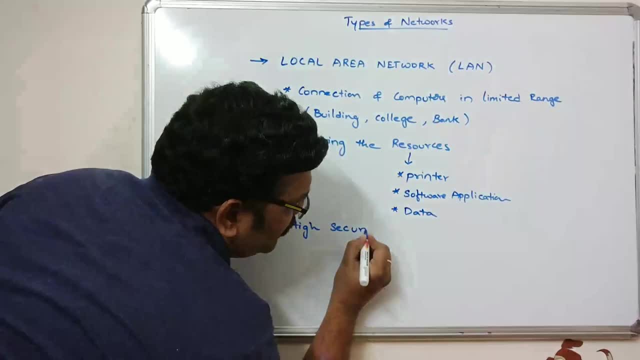 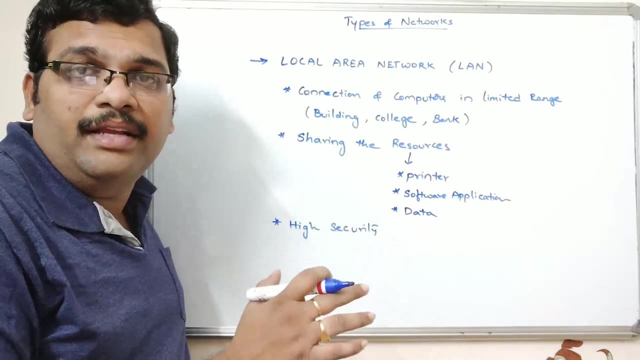 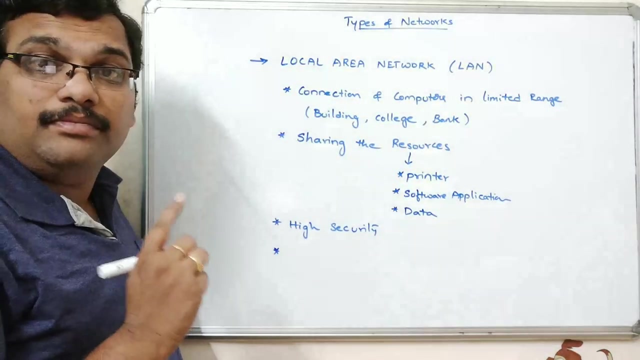 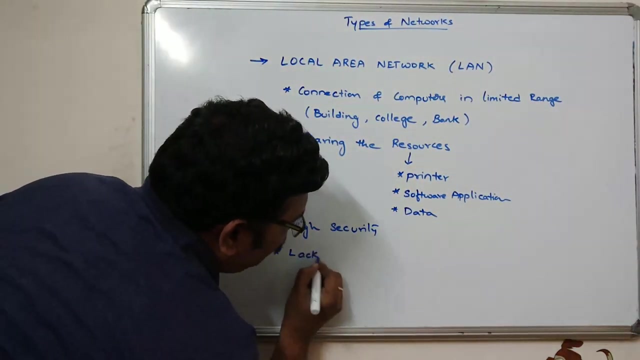 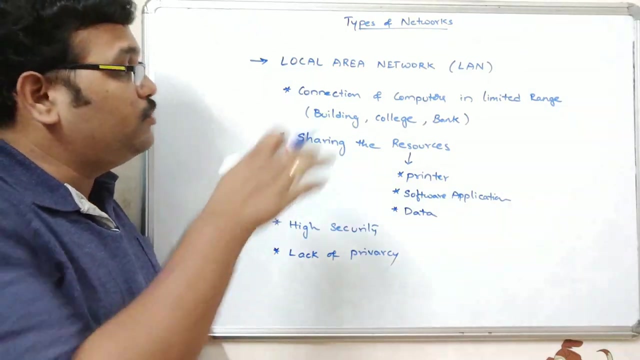 it is, it will be having high security. okay, because there will be a limited number of computers and the range will also be within the- within the limited range, so we can achieve the high security, but but lack of privacy, so there will be no privacy. once a data is used in the system, that data can be accessed by all the users of a local area network. 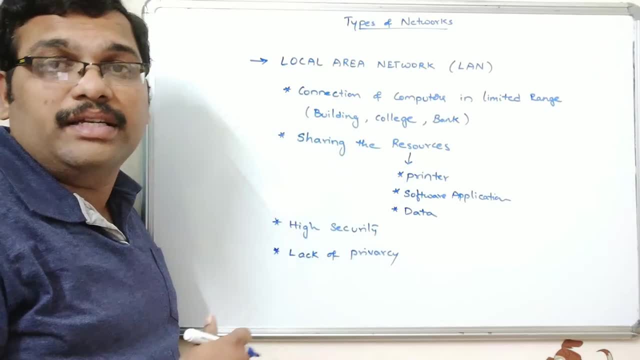 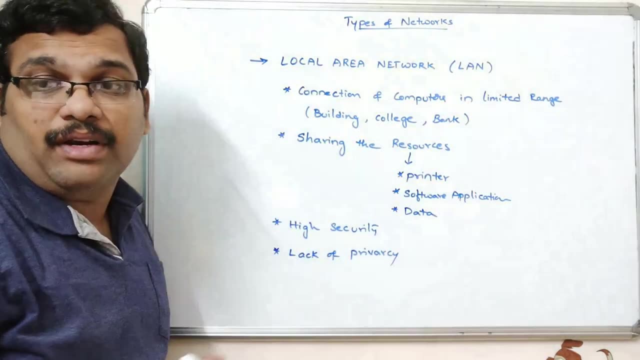 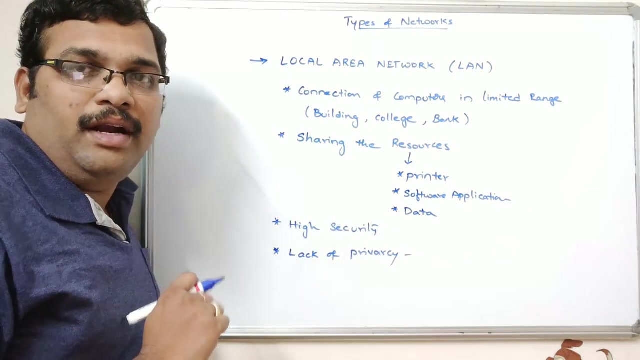 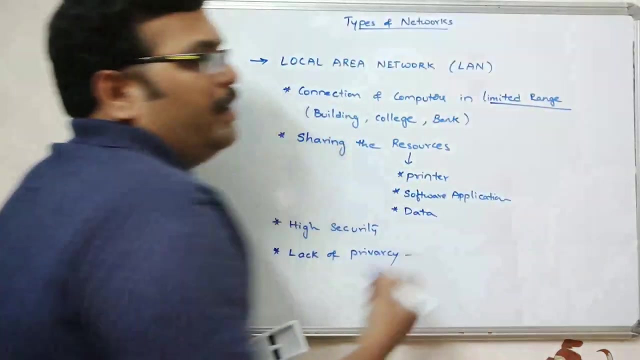 so a data can be accessed by unauthorized users. unauthorized users means all the users which are available in the local area network. so that is main drawback of this local area networks, right? so hope you understood this one. so main purpose is: within the limited range this will be: 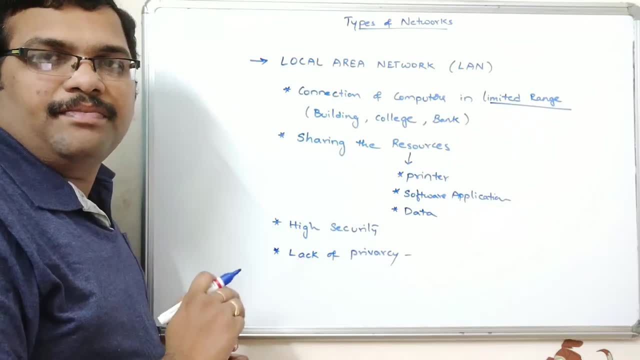 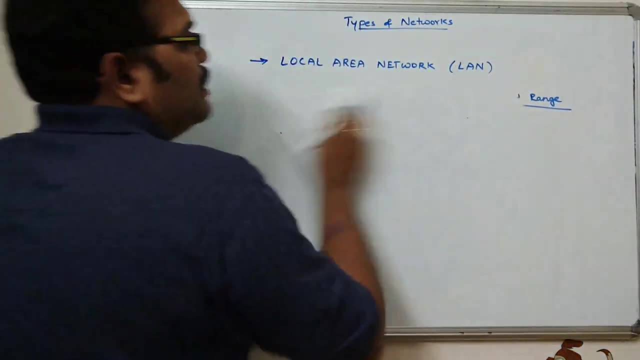 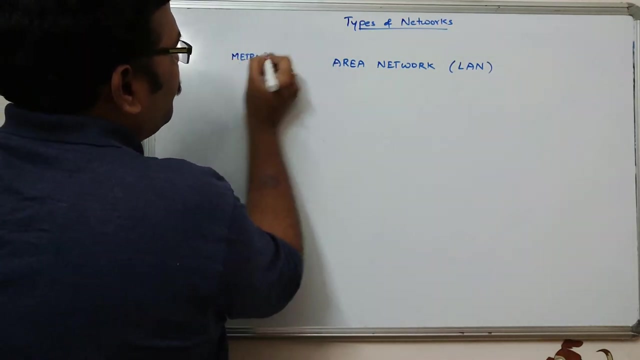 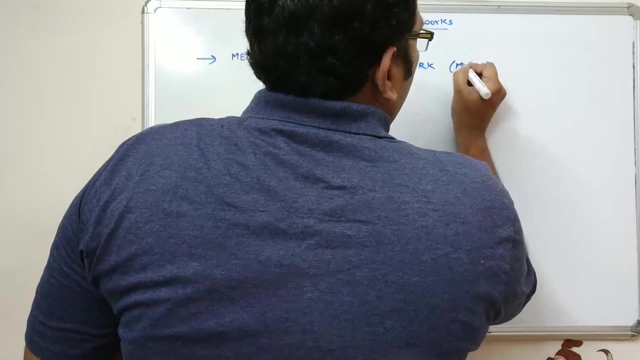 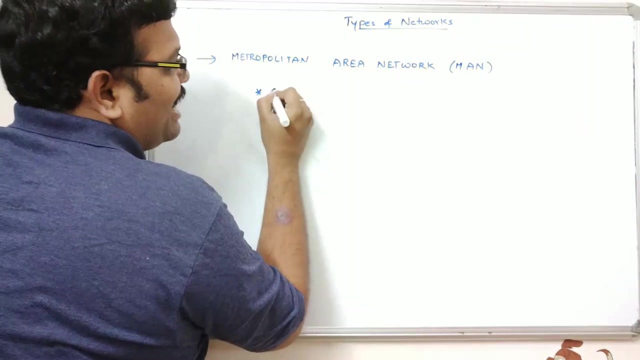 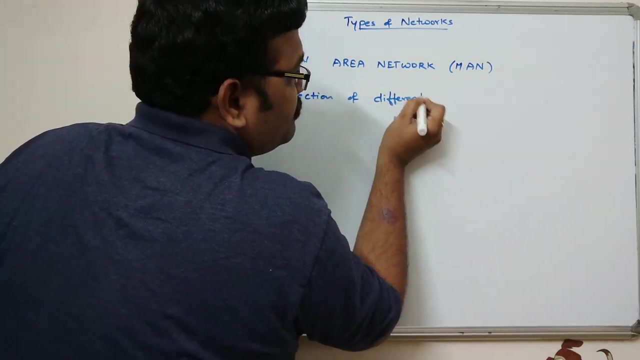 established in within the limited range. all right that within the building or a college or a bank. now we'll go with the second type of network, that is, metropolitan area network. so this is a common area, so we know that that. so that is a common area. this is commonly known. 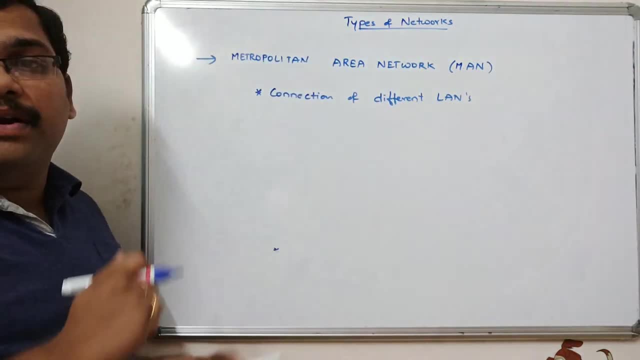 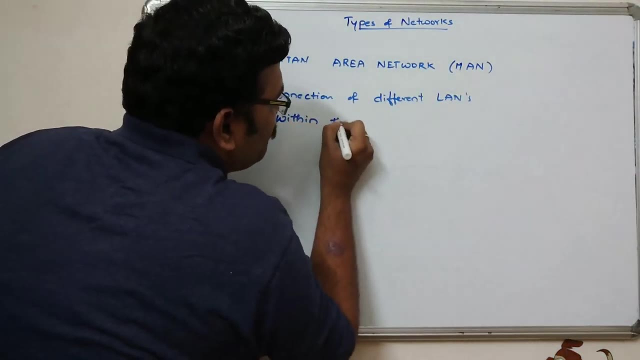 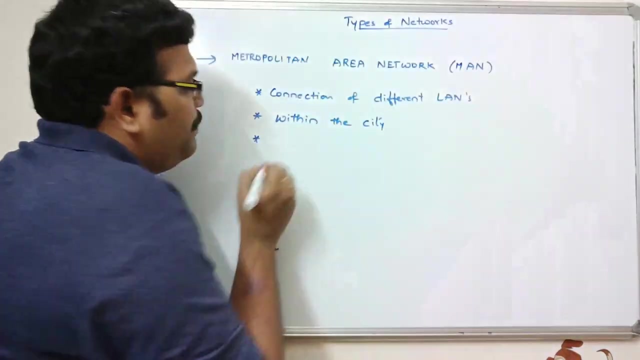 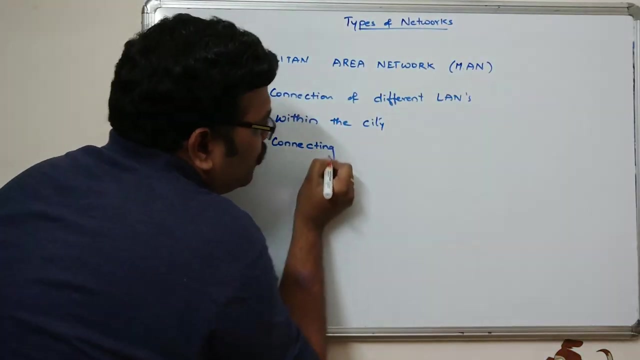 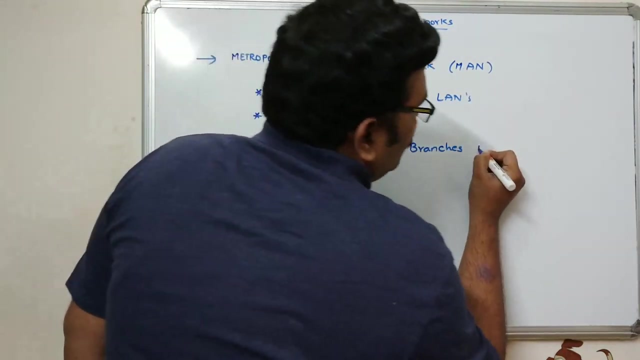 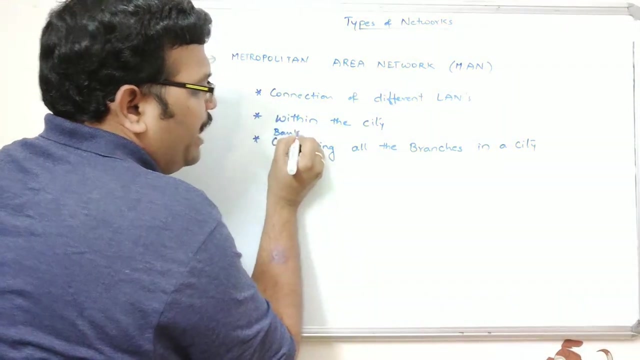 see, this is commonly known as man metropolitan area network, so it is a connection of. it can be connected within the city, within the city, right? so an example. so example means connecting all the branches in a city. so if you take any bank, okay, any bank. so connecting all the branches in a city. 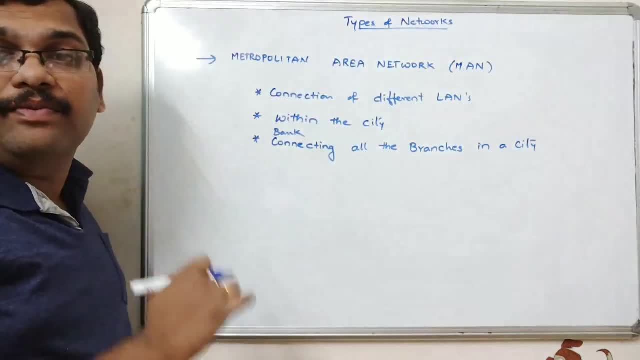 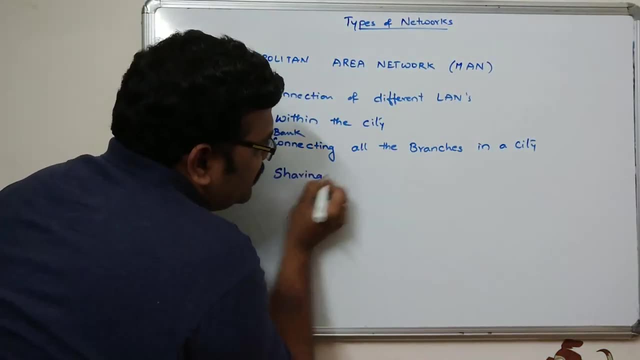 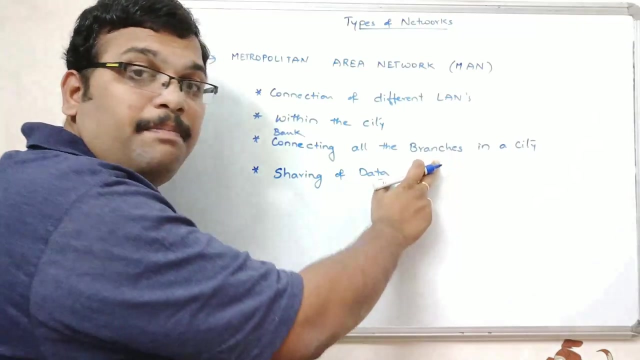 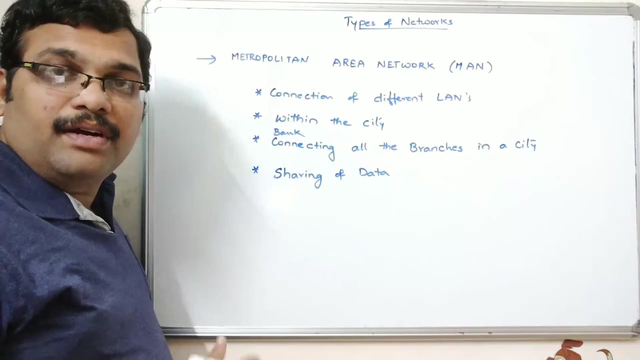 will be considered as a metropolitan area network. so the main purpose of this connection is sharing of data, sharing of data, so the data will be centralized, so that any branch, any branch, can access the data right. so this is one best example for this, this one. so again, 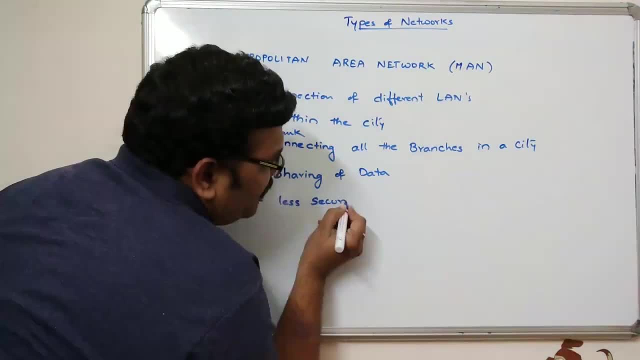 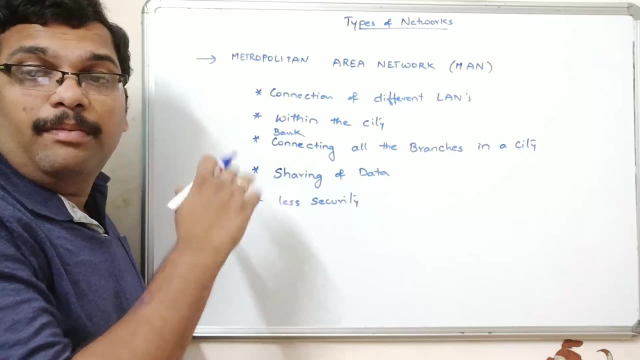 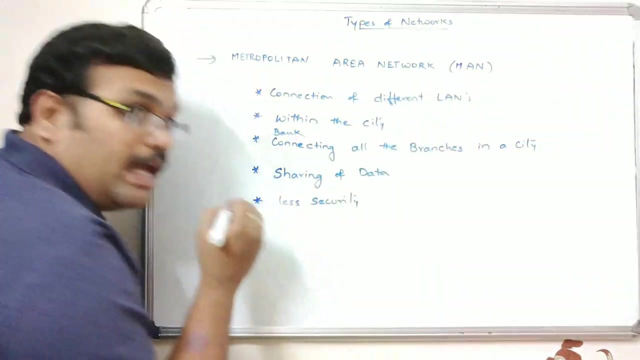 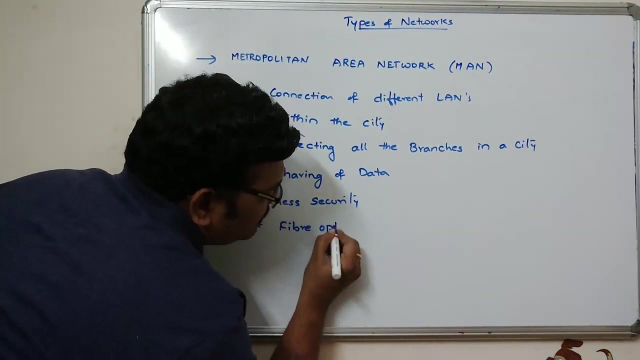 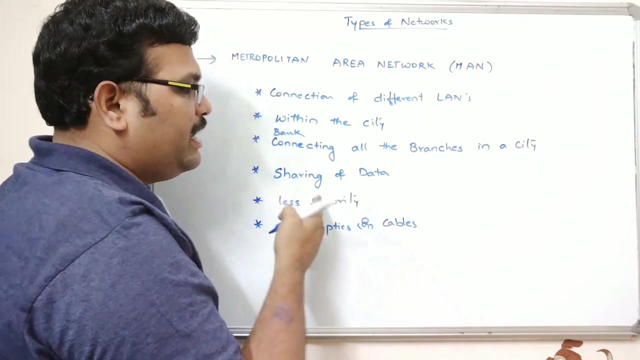 it is also having the less security because multiple users will be accessing this one, so it will be having less security. and these LANs will be connected with the help of fiber cables, fiber optics or cables, so with the help of these transmission media, the data can be shared from one branch in a city to 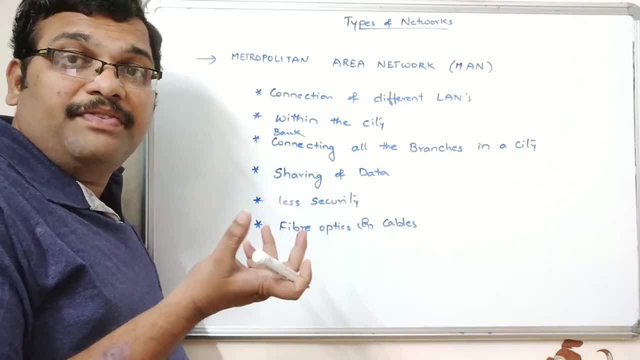 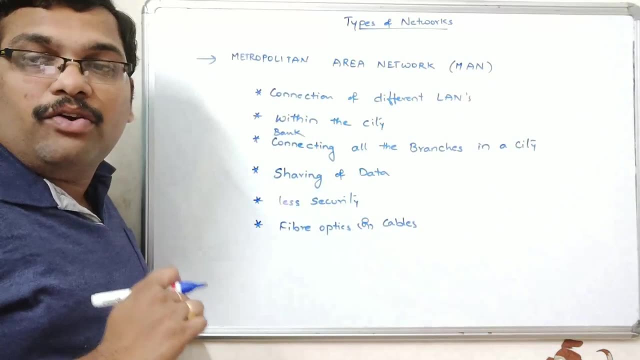 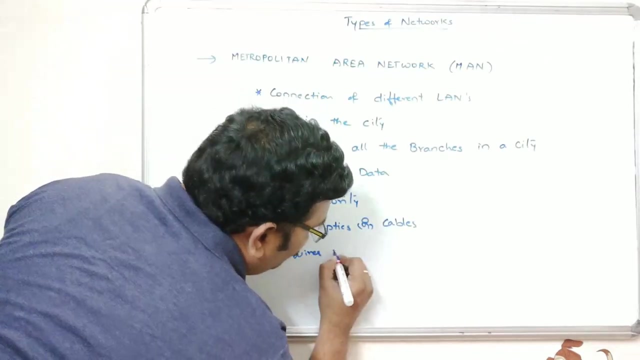 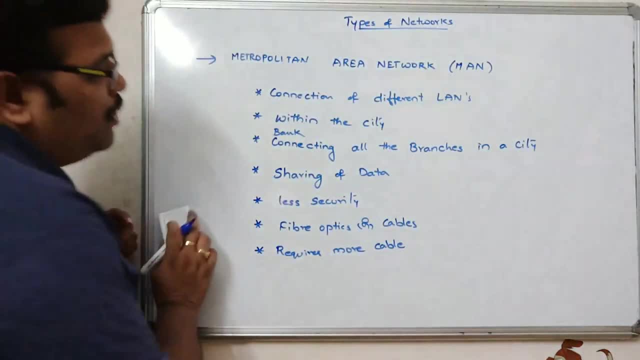 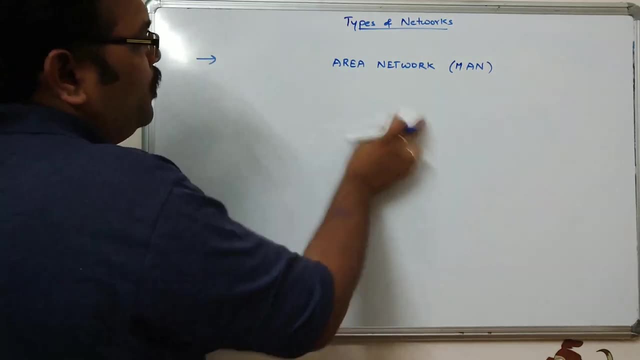 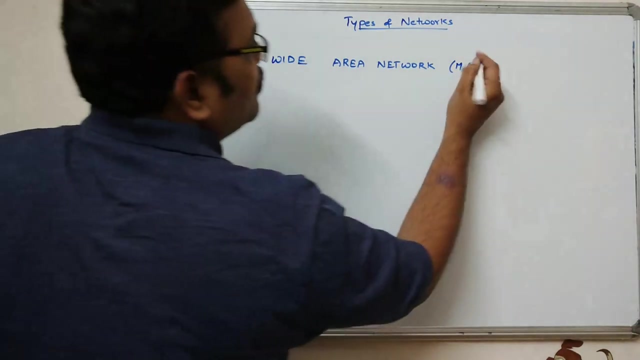 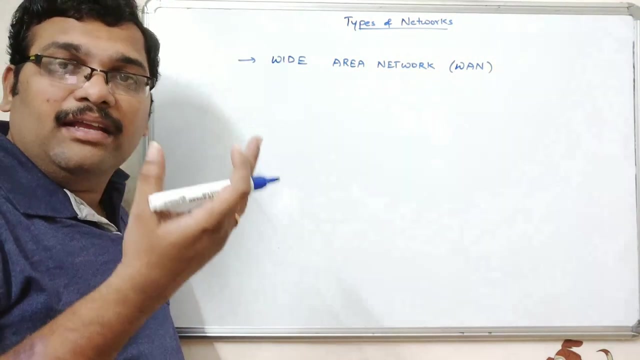 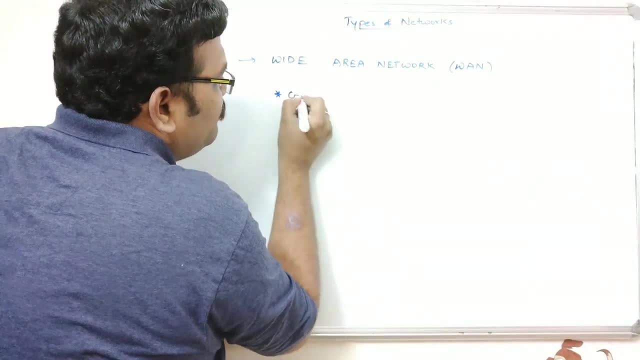 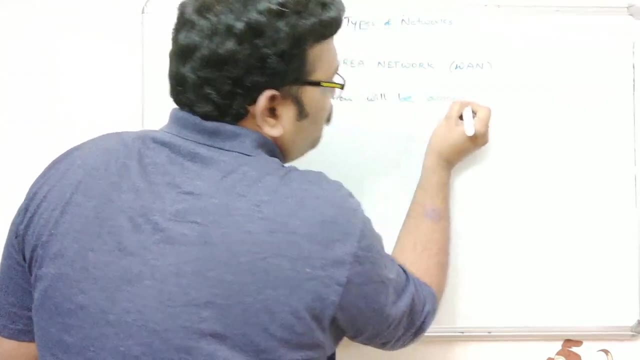 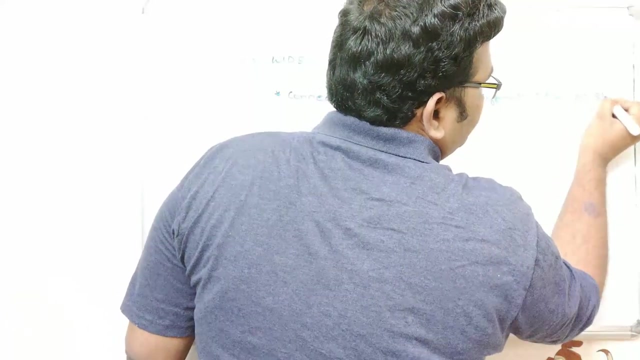 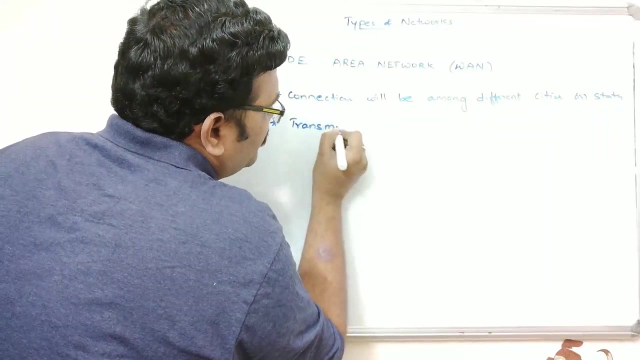 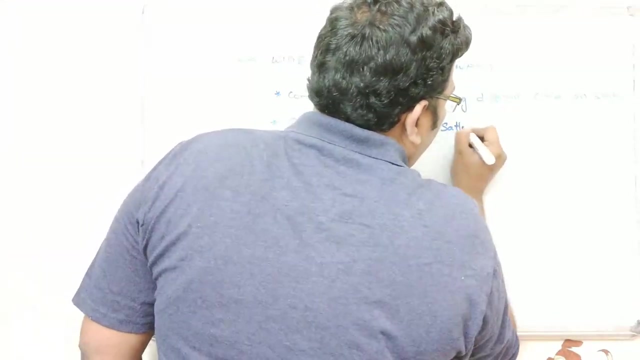 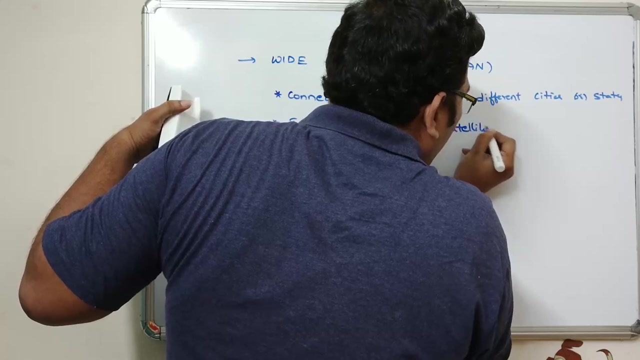 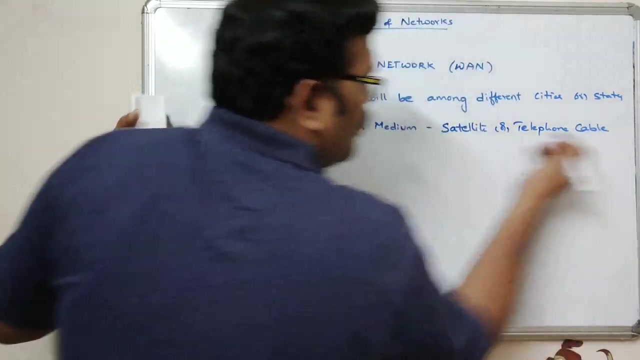 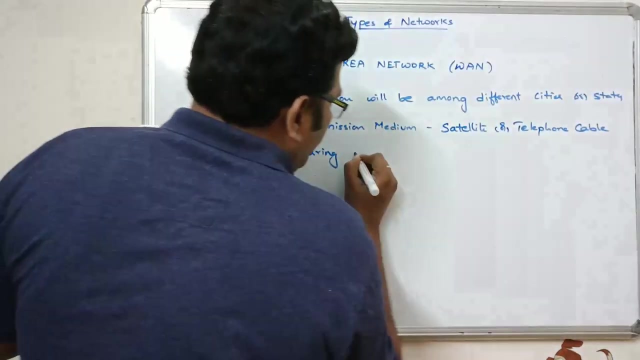 different cities. okay, here the connection will be among different cities or states, and here the transmission media is see. here the transmission media medium will be satellite or telephone cable, and the main purpose of this wide area network is also sharing of data and it is a connection of 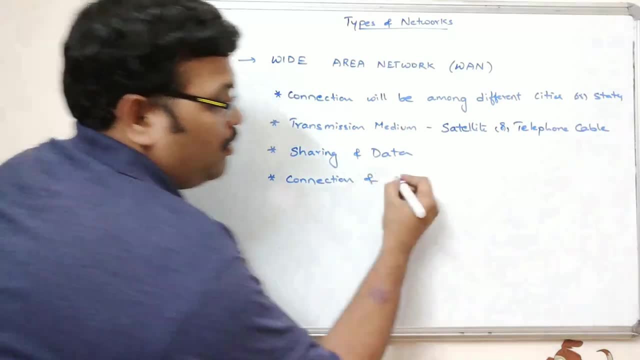 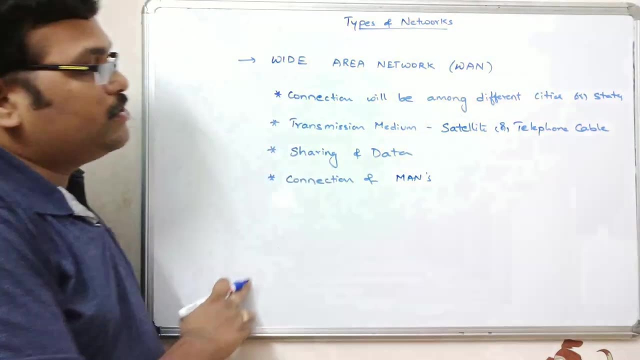 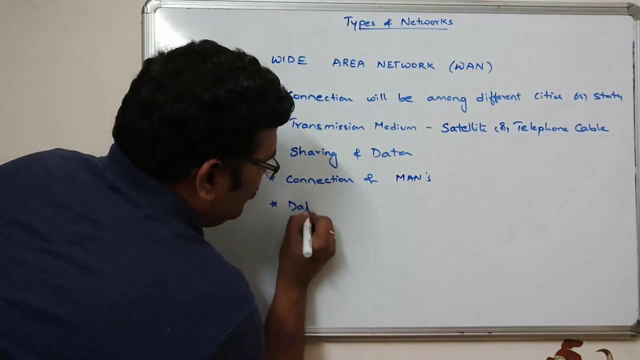 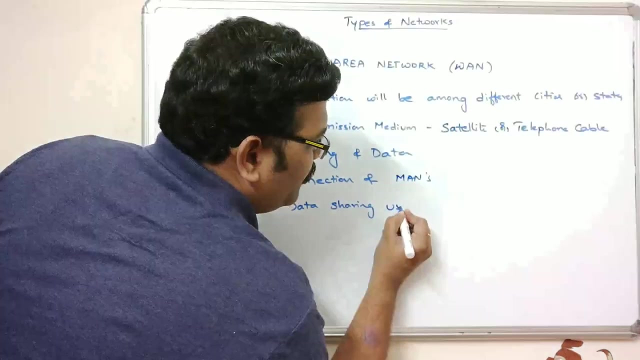 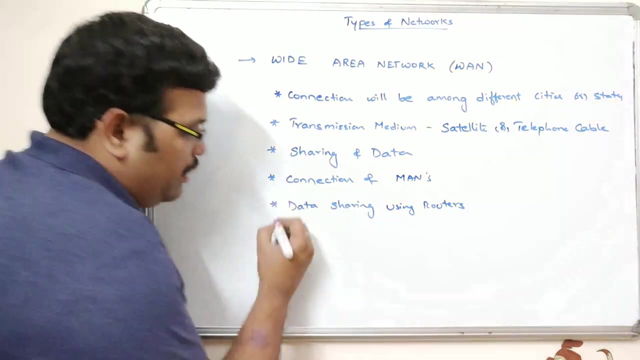 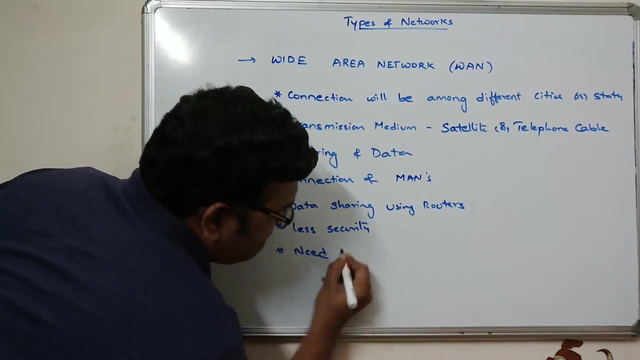 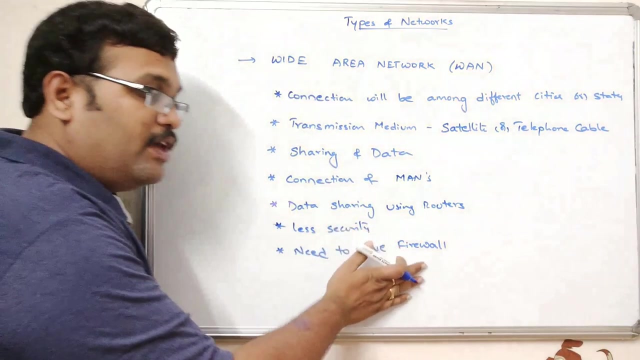 it is a connection of mass by metropolitan area networks. so here, with the help of routers, the data is shared. data sharing will be done with the help of this telephone cable or a satellite, using routers. routers right here also will be having less security, need to have firewall, need to have a firewall in order to restrict. 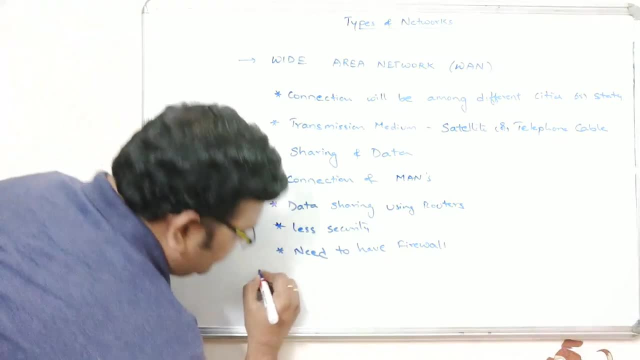 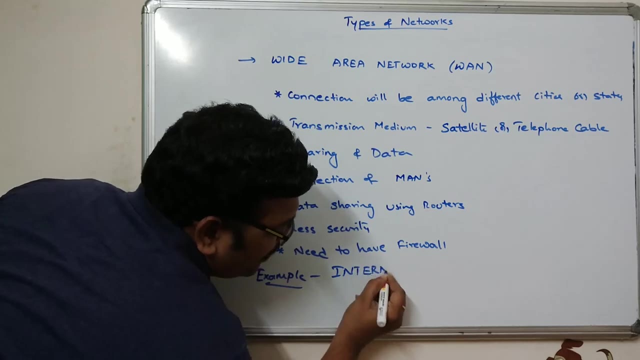 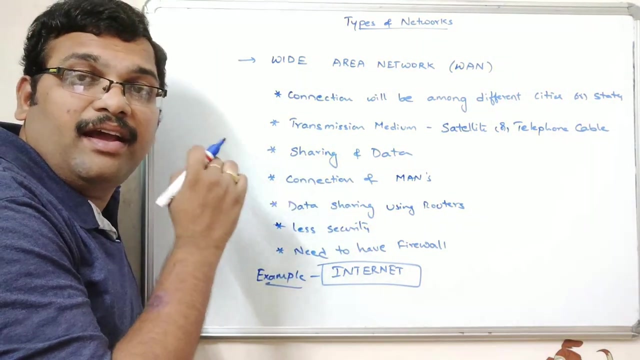 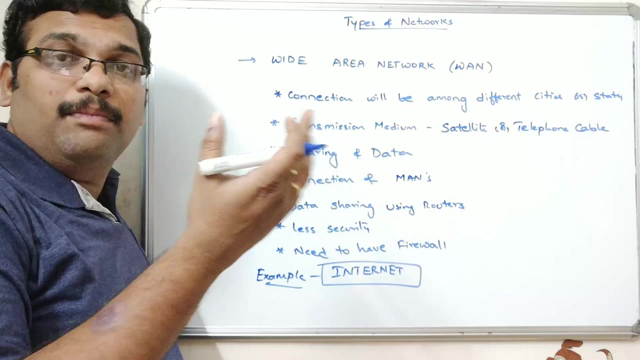 the authorized access to this one and best example for this wide area network is internet. it's a world wide web. internet is a best example for this wide area network. so by using the internet we can share the data from one computer to another computer which is available in different states or different cities or different countries.